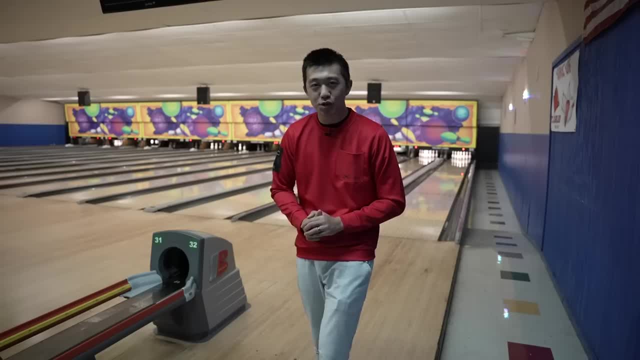 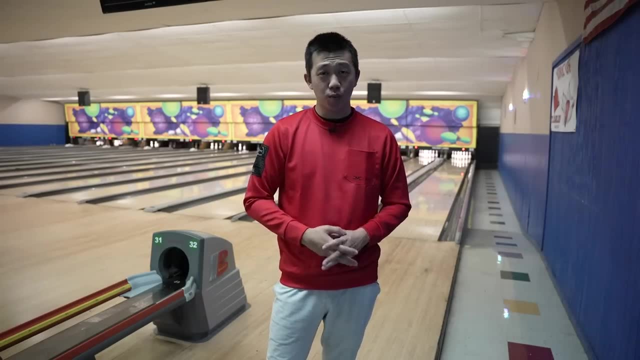 this year on tour, 14 pounds has kind of been the talk of the town, starting with Bill O'Neill. He went to 14 pounds earlier in the season, switched back to 15, but a few other guys are doing it as well: Tom Doherty and most recently you probably heard, if you watch the PBA league, Ryan Simonelli. 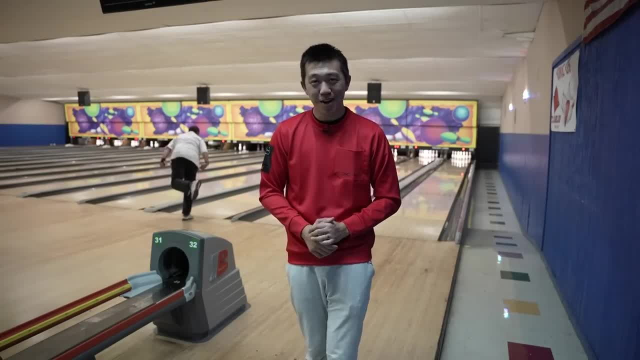 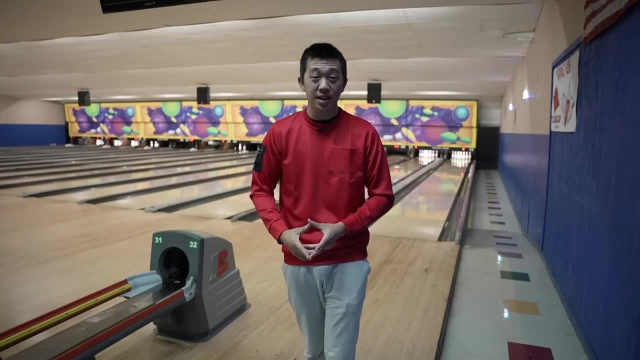 His ball is hitting pretty hard. and that was 14 pounds. So I said, hey, why not, let's order a 14 pound TNT infused and let's give it a try. But the reason why I chose the TNT infused is because there's the biggest disparity in the 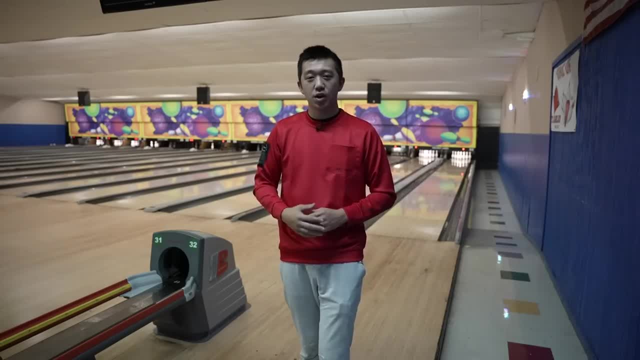 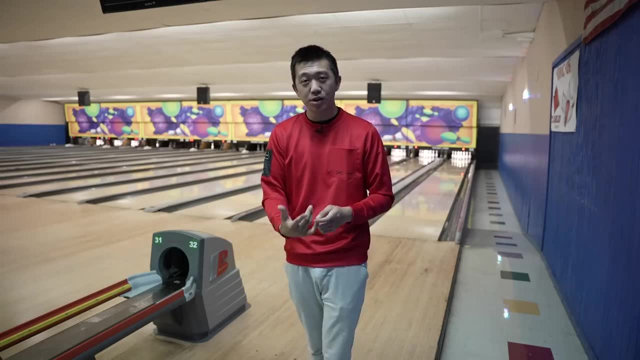 RG numbers between 14 and 15.. So I believe the RG for a 15 pound TNT and TNT infused is 247, whereas the 14 pound is all the way up at 254.. So that's seven points different. That goes from mega low RG, which 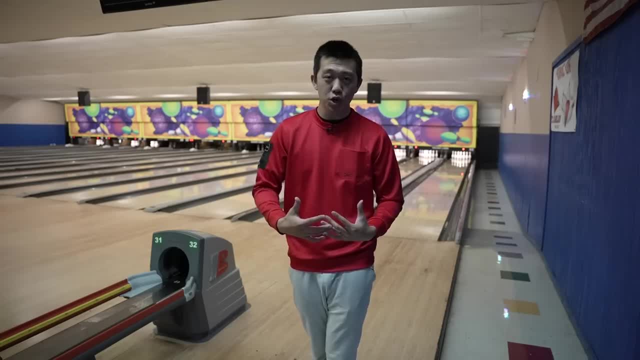 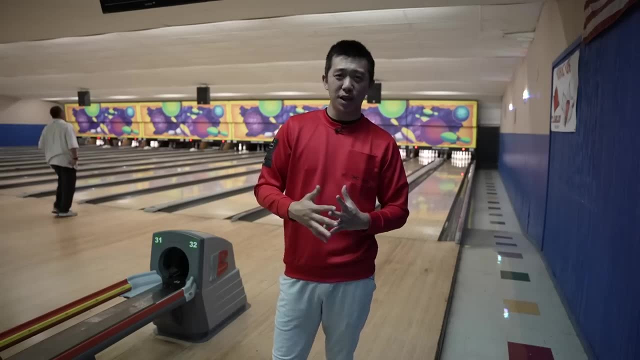 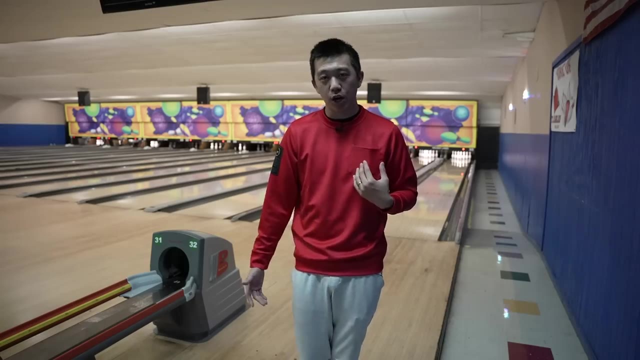 for those of you that don't know, that helps the ball get reading much sooner. all the way up to 254, which is pretty mid, almost high RG, The numbers for the 14 pound get pretty close to like a 15 pound Revenant, which is a ball that I throw pretty much later in blocks when they're really hooking. 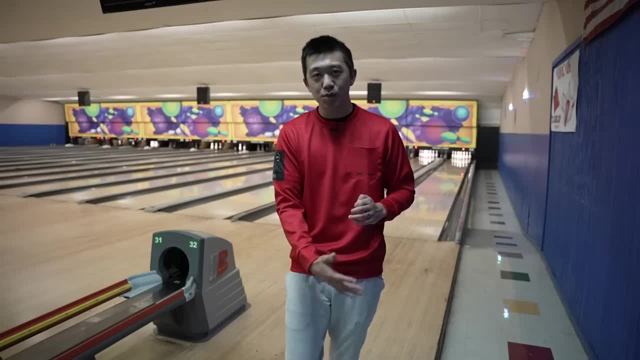 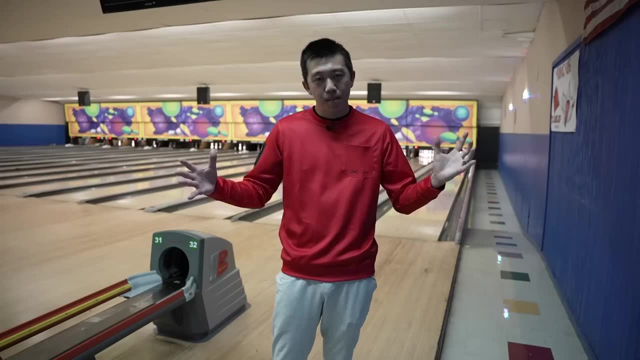 So very interested to see, especially here at Holiday Lanes where they hook a good amount, and these lanes are already pretty transitioned. You're going to see a pretty big difference in the shape. but I'm going to get into the bowling and you guys are going to watch, So hope you enjoy. 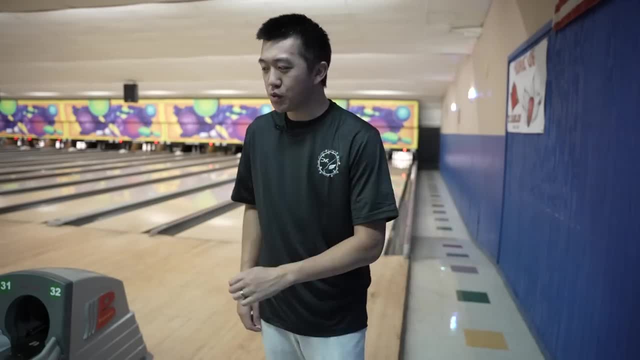 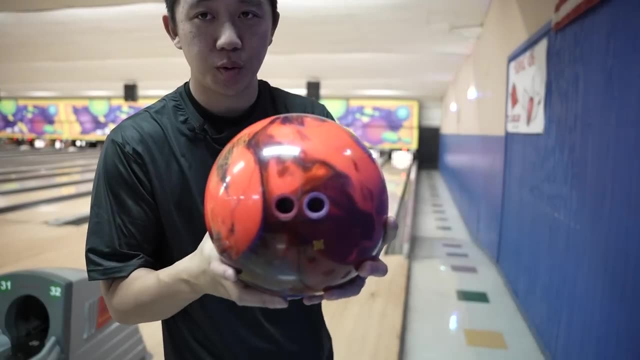 Alrighty guys, I'm going to start with the 15 pound TNT infused. Obviously it's a ball that I've already thrown, Has not too many games on it Again, like I said, five and a half, two and a quarter buffer pins tall over my middle finger. 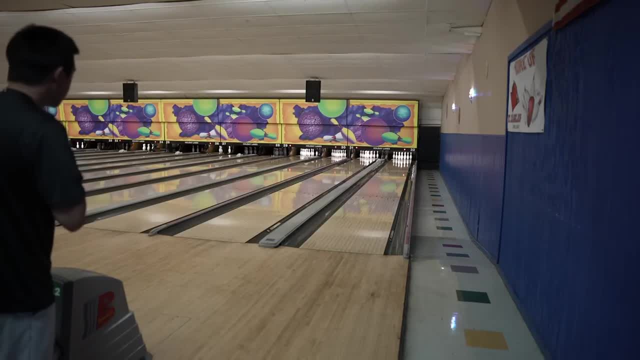 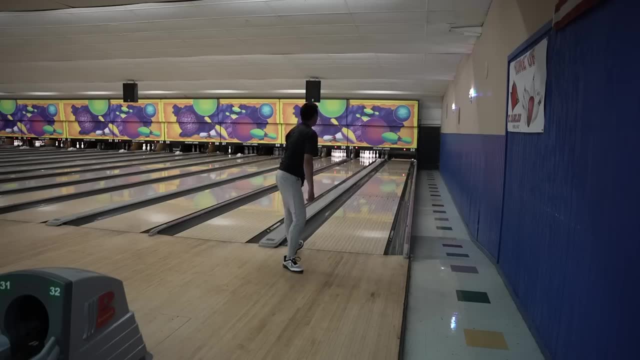 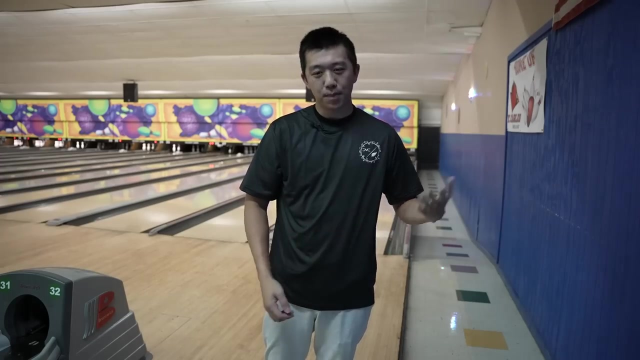 Like I said, these lanes are pretty transitioned, so that was a pretty terrible shot. As you can see, since these lanes are broken down a lot, that ball kind of used a lot of the energy in the front. It wasn't as boomy as, say, the strike challenge video I filmed, but I'll throw another one. 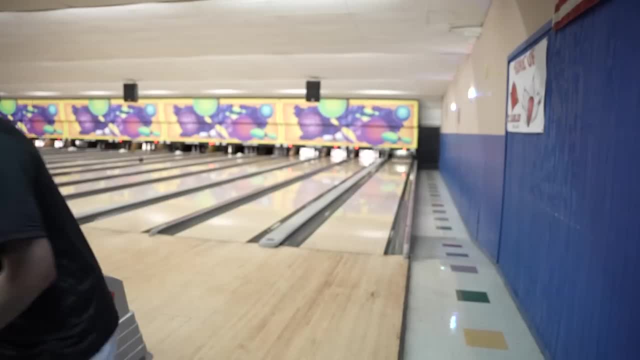 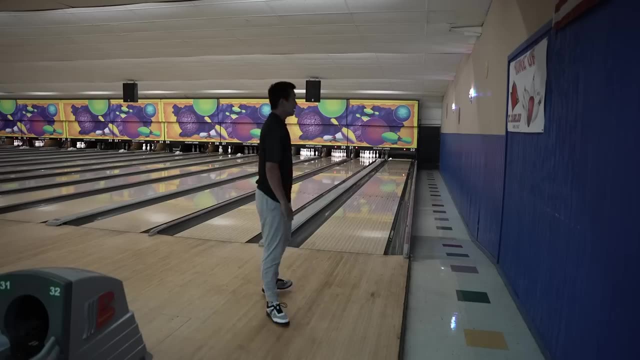 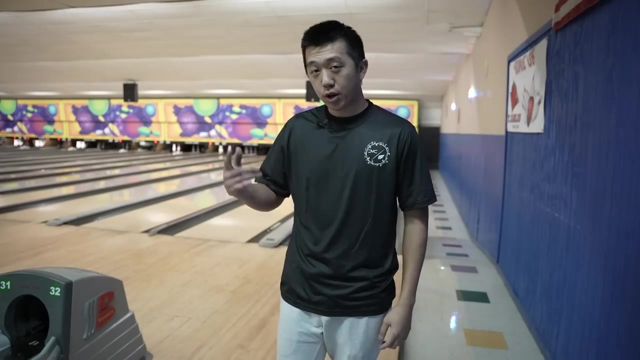 Hopefully better. Another shot to the friction and then we'll go to the 14.. Yeah, it's getting going really forward, just because that super low RG is getting to pick up pretty early. But we're going to go to the 14 pound. This one I threw a couple times and 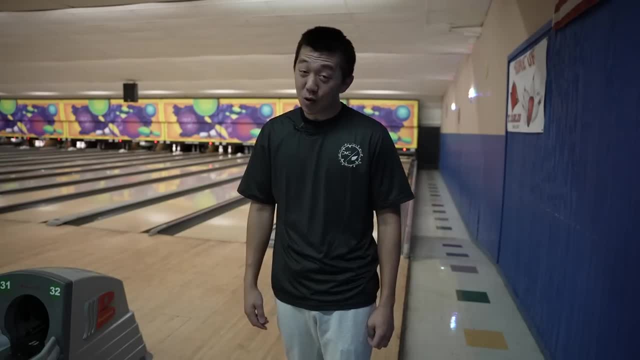 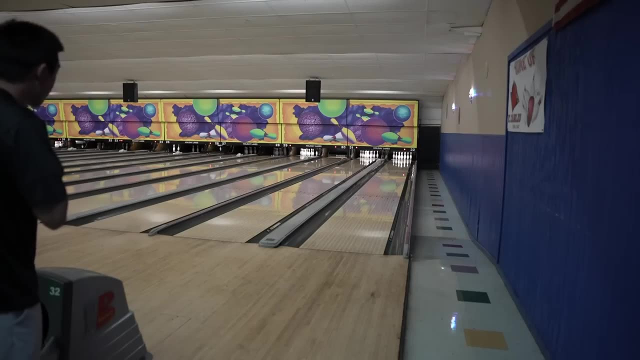 those seven points of RG make a lot of difference and you're going to see why. and then I'm going to explain why, Standing in the same spot, I'm going to do my best to release the same. Honestly, my rev rate does get a little higher with 14.. 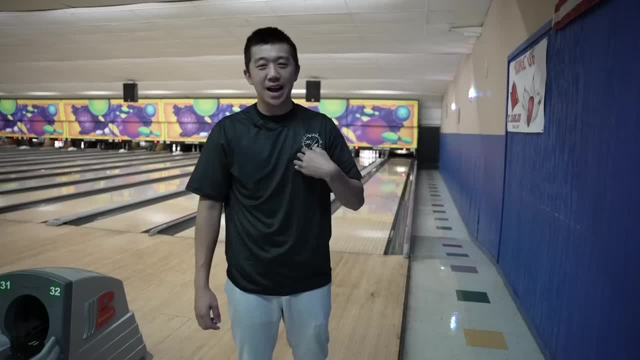 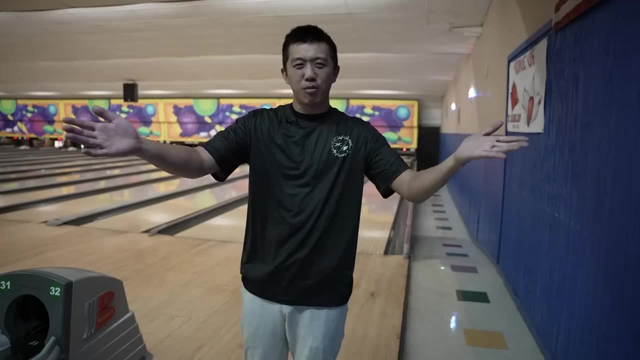 That was also a pretty terrible shot, but I don't know if you guys could see it. I can see it. It's quite a bit quicker off the friction. That's because it's just retaining way more energy in the front part of the lane. I'm going to try and get one remotely close to where I'm supposed to be. throwing it, and then you guys are just going to see it. I'm going to try and get one remotely close to where I'm supposed to be throwing it, and then you guys are just going to see it. I'm going to try and get one remotely close to where I'm supposed to be throwing it, and then you guys are just going to see it. 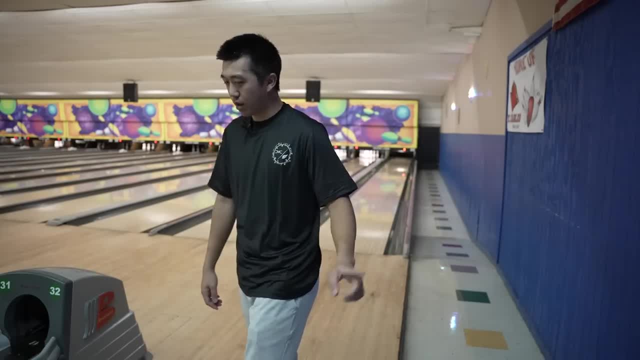 I'm going to try and get one remotely close to where I'm supposed to be throwing it, and then you guys are just going to see it- Big old hodgepodge of shots after this. So I'll throw one more and then we'll get onto it. 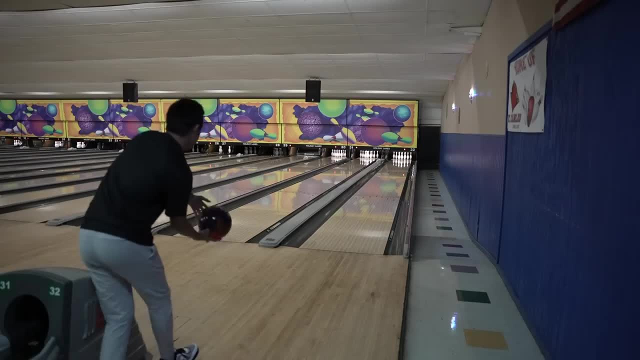 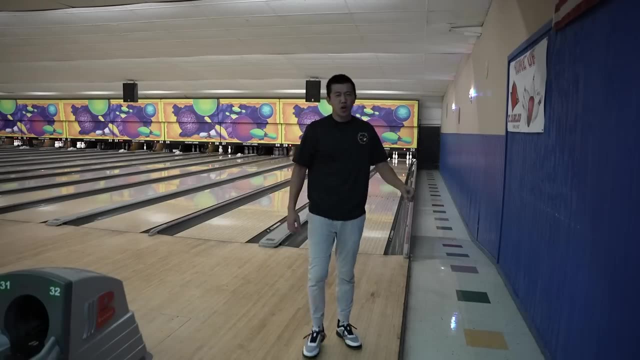 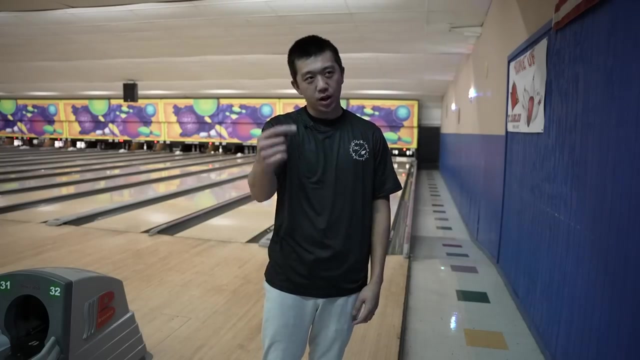 Alrighty, hopefully a better delivery here, That's better. See, that was almost in a similar spot to that first shot. I threw with the 15 pounder and it just it's responding to the friction so much faster and that one got going to a. 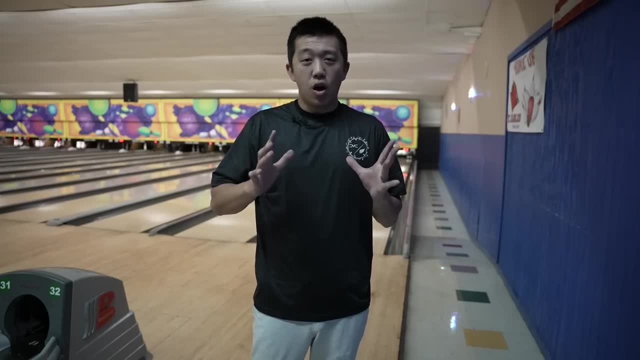 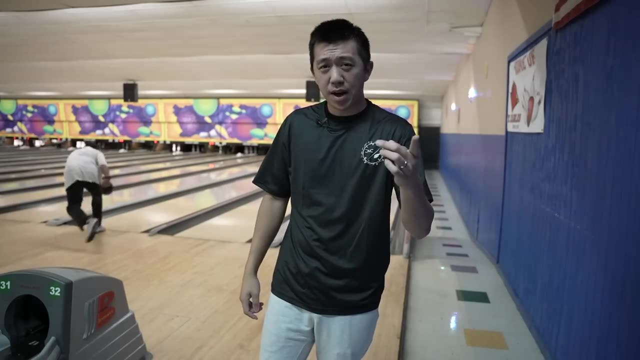 big four. So I will say that all of the numbers don't change the same when you go to 15 pound, 15 pounds, 14 pounds. So definitely come into TV Bowling Supply and talk to us about it If you're considering a 14 pound change. 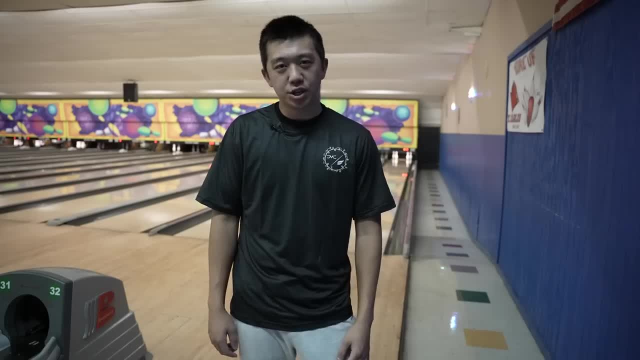 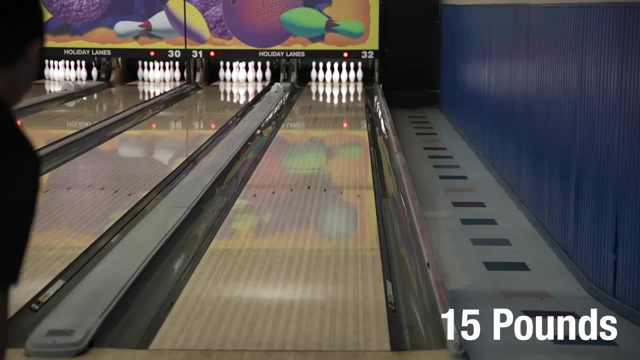 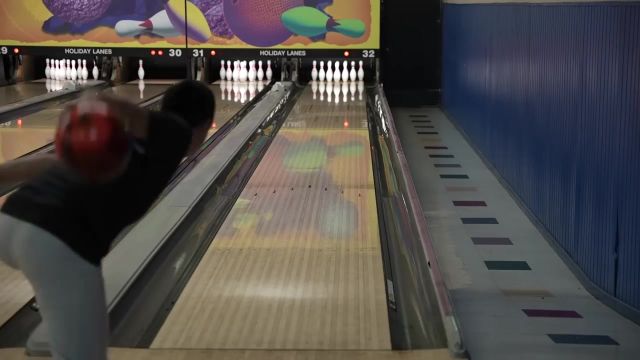 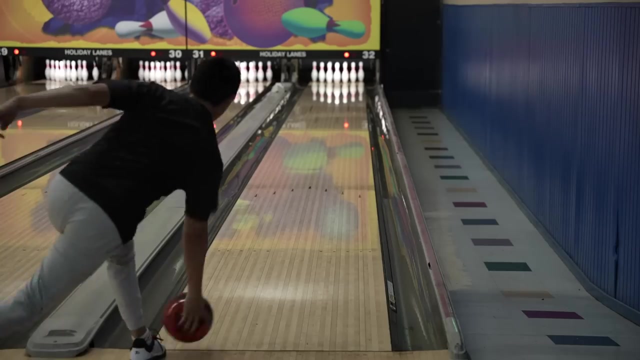 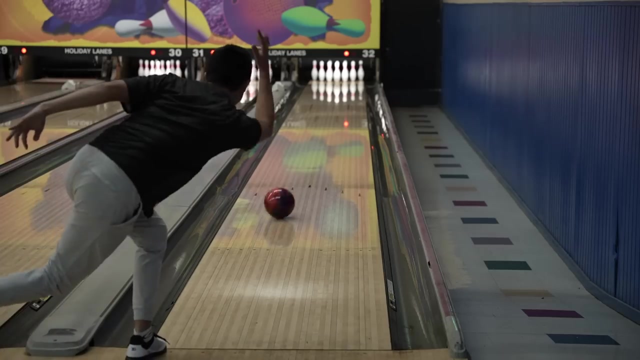 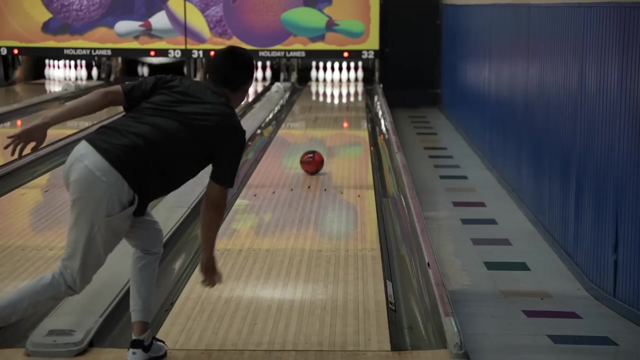 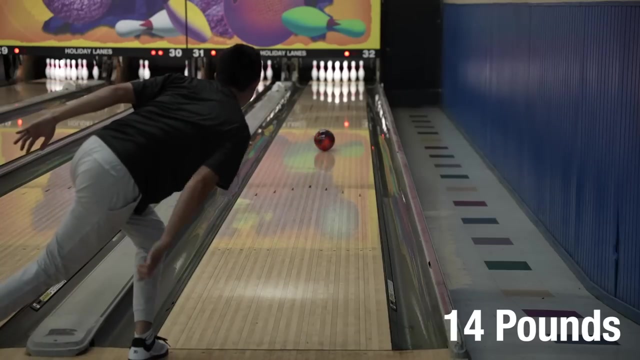 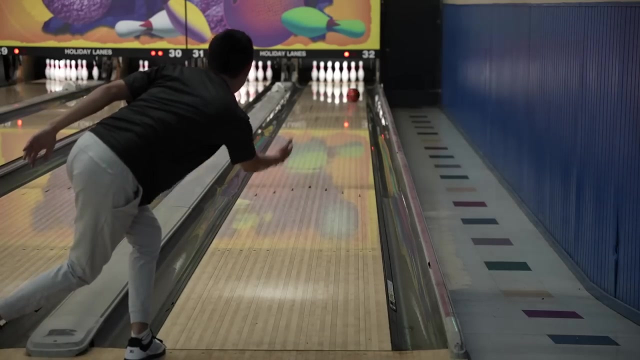 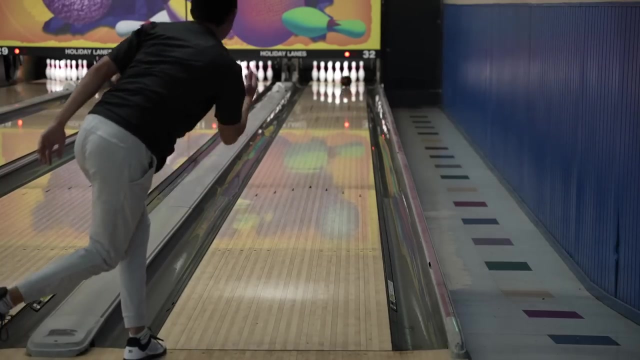 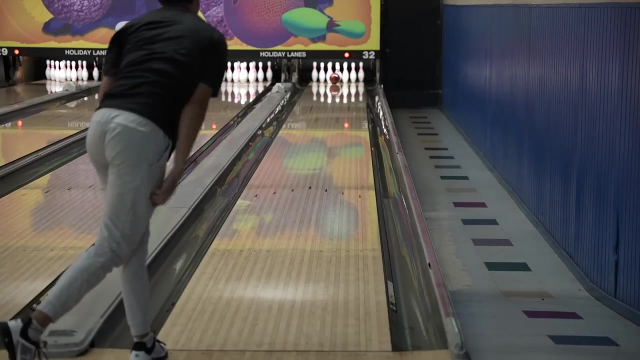 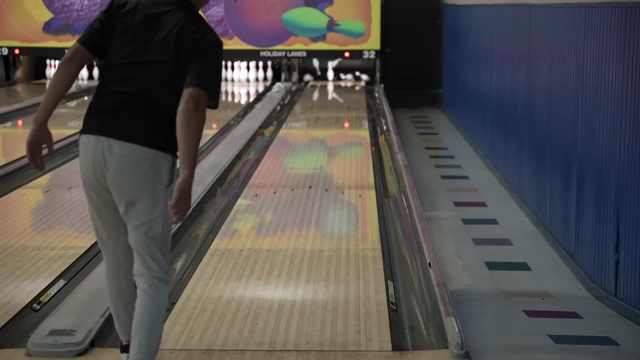 but I'm gonna show you, guys, just a bunch of shots with each of the 14 and the 15 pounder, just so you can see the difference And then talk to you more about it after All. right guys, there you have it. 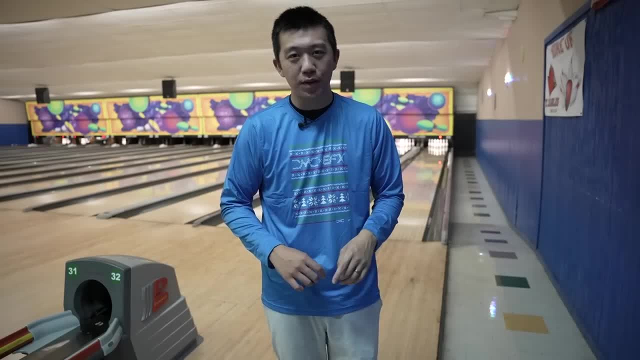 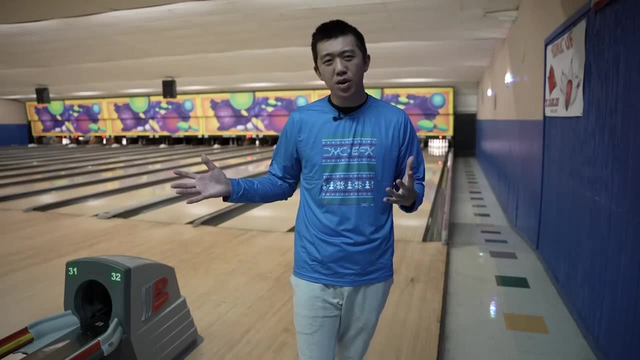 There were five shots with the 15 pounder and then five shots with the 14 pounder. I don't know if you guys could see the difference as much as I can Cause honestly, bowling balls are 80, 85% cover stock. 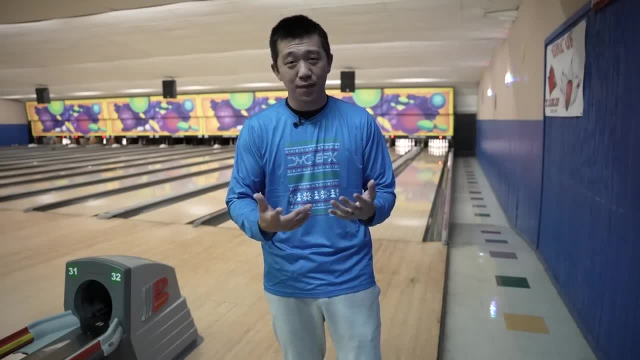 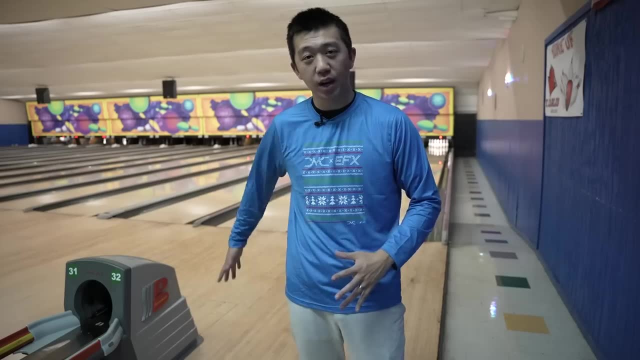 as far as ball reaction, But the trained eye can see that 15 to 20% And the biggest kind of difference I saw with those two is, like I said earlier, the 14 pounder retaining way more energy. As you can see, the one shot at big forward. 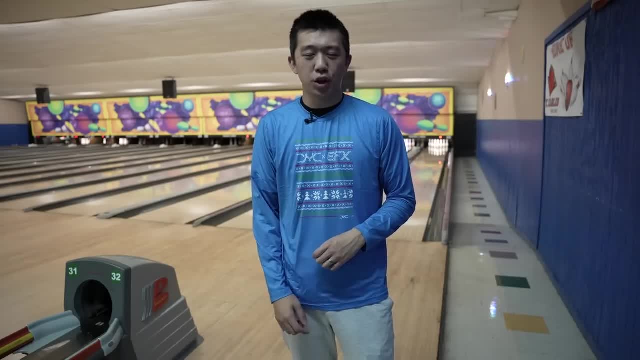 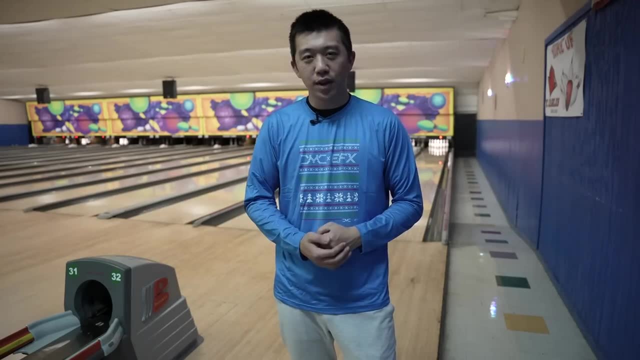 And that was just cause where the 15 pound was kind of blending out the front a little bit better. The 14 pounder retained just enough energy to get offline And also when the 15 pounder left that flat 10, I just don't feel like that 14 pound is going to at this time. 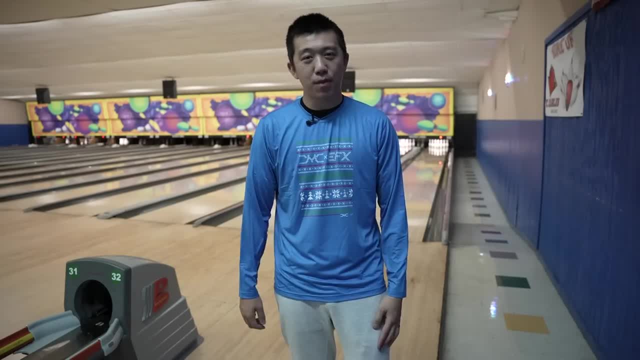 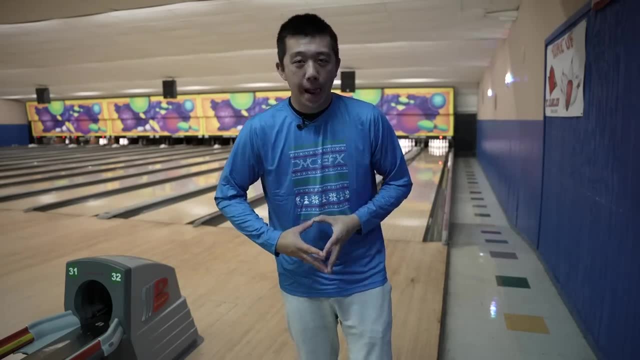 Just because, like I said, it's retaining that much more energy in the back by the lane. As far as the TNT infused is concerned, very big difference. But, like I said, go talk to your local Storm VIP pro shop- hopefully TV bowling supply- and talk it over. 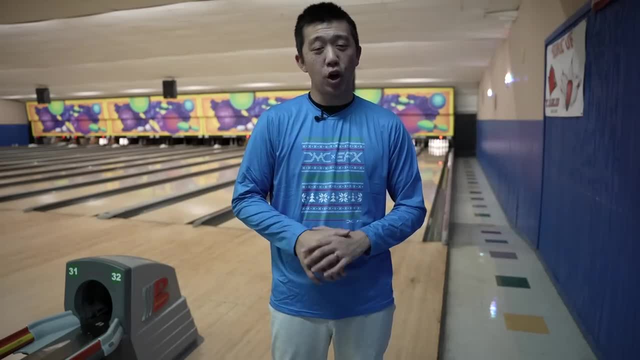 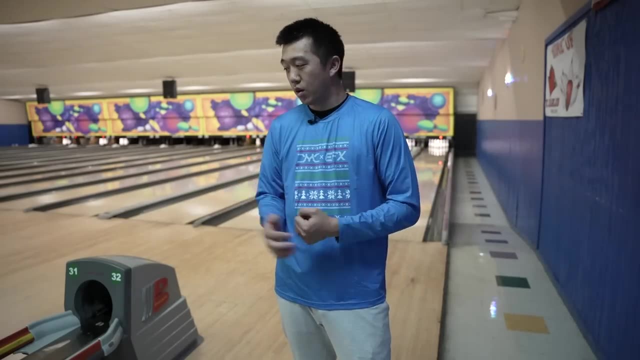 Cause I know some other balls- the difference isn't as great, or even there at all. Like the summit, I think the numbers stay exactly the same, But some change by two, three, four points in RG, or some change by seven, like this ball. 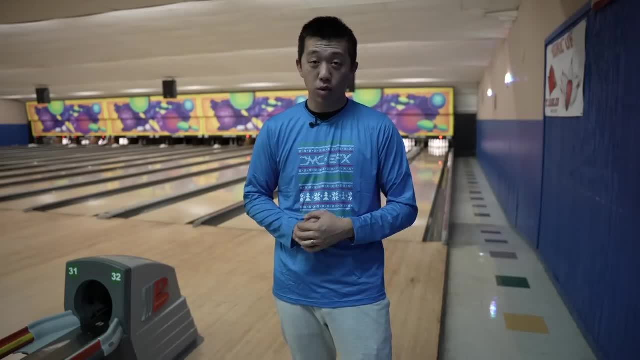 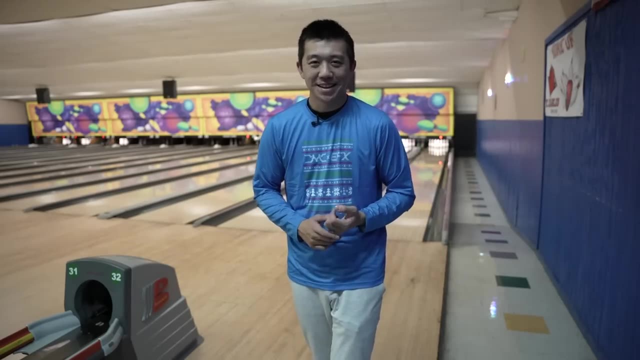 So definitely something to discuss with your local pro shop. This is definitely an interesting experiment for me. I didn't think I would even consider going to 14, but after throwing this TNT I might. It is much easier to throw. The river rate does go up a little bit. 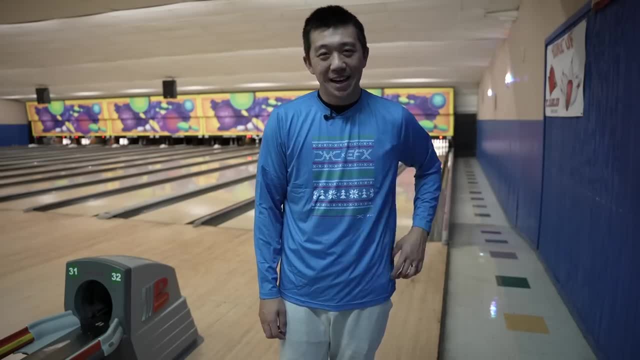 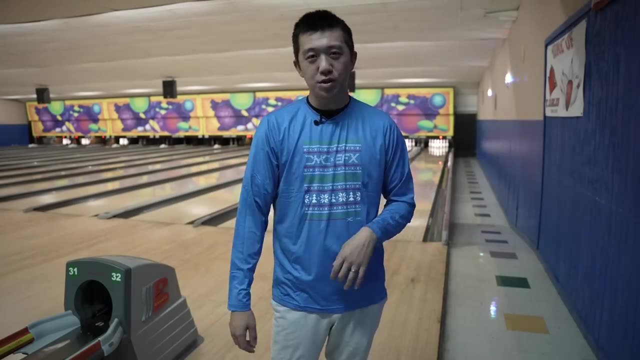 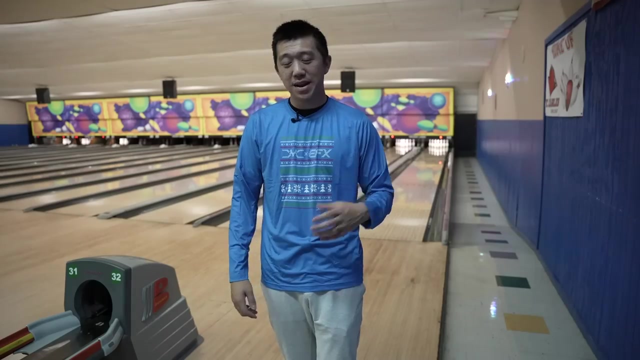 So that's something, but it's very interesting And I think since bowling balls have dynamically changed so much. back when they were just three piece balls- pancake weight blocks- all you really had was that static weight, So a lot of people were throwing 16 pounds back then. 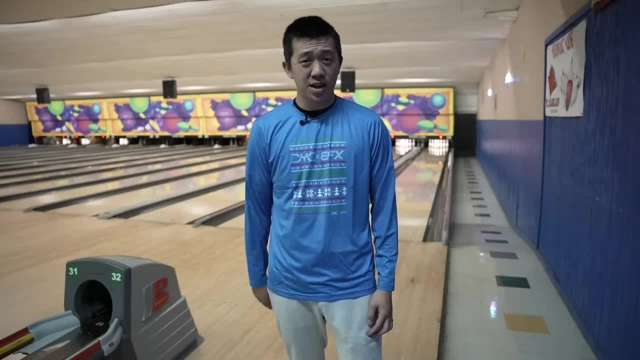 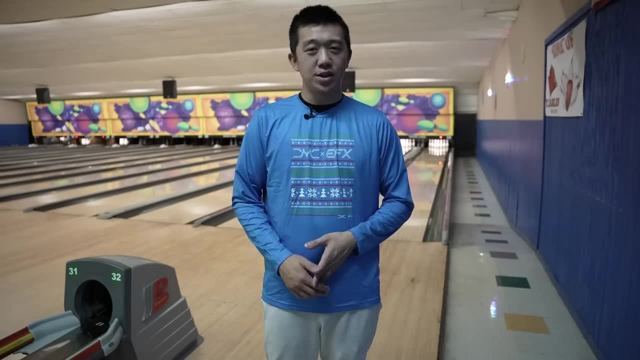 but now you can back down to like I showed you 14 pounds and not really lose much. It's a little bit easier on your body And the balls are just so dynamic. now There are more factors other than just the static way. 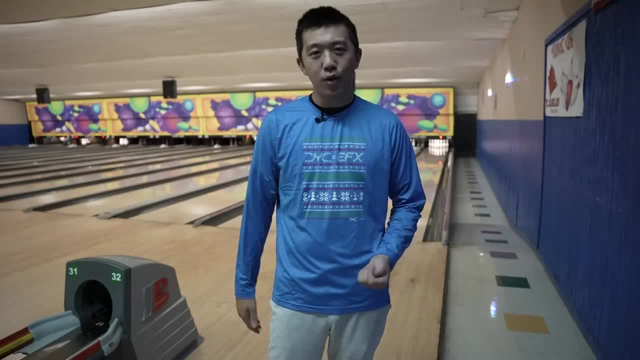 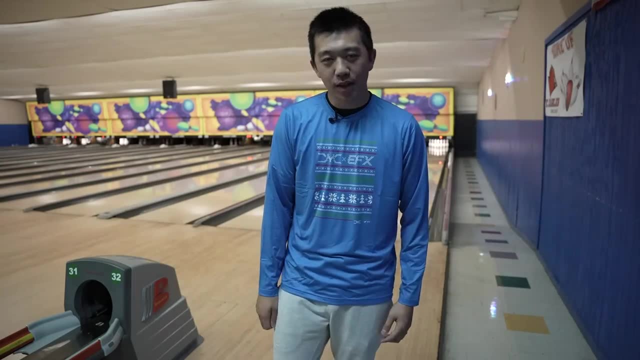 of the bowling ball that kind of contribute to that hitting power, or I don't know what the scientific term is: kinetic energy, whatever. there are ways to create that other than just the way of the bowling ball. So thank you guys again for watching. 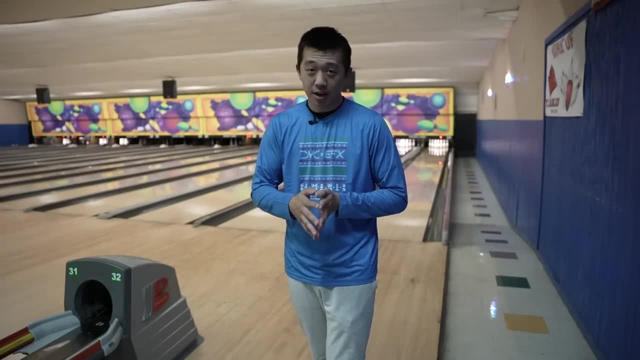 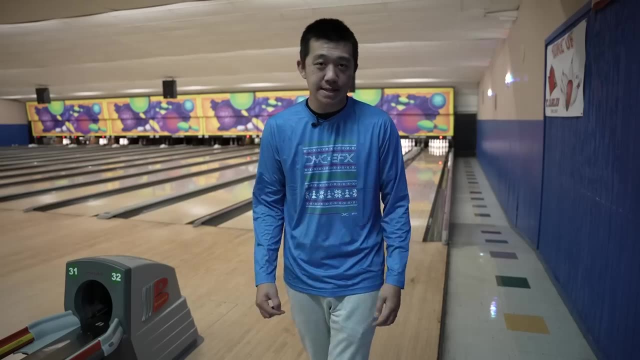 I hope you guys enjoyed this episode of Ballsplanations. Let me know down in the comments below what other topics you want me to hit on and I will get right to it. And if you did notice, I hope you noticed. if not, then I don't know where your focus is. 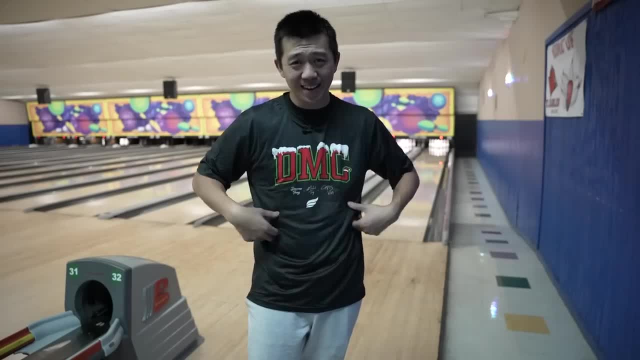 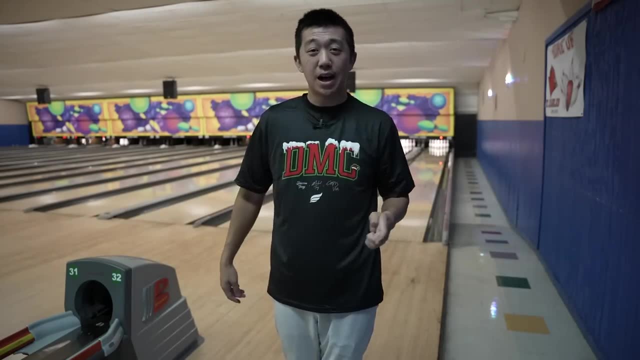 I've been changing shirts. just like this. bang, just like that. This is our winter, or for Christmas: Bold DMC drop dropping December 1st. I'm assuming pre-orders are gonna happen sometime in November, so go and follow. 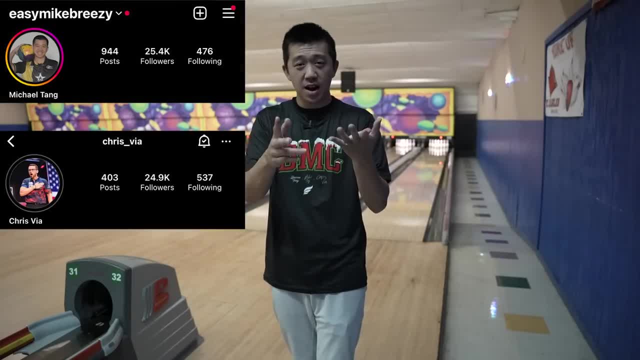 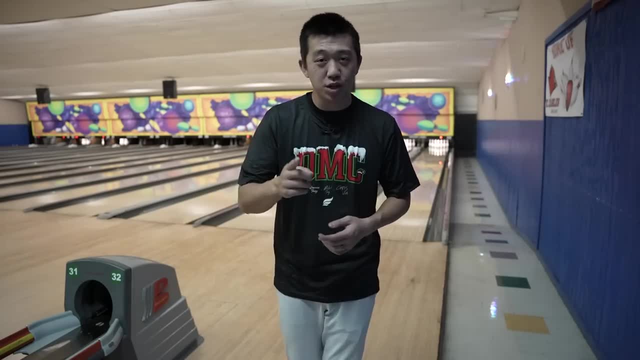 my personal Instagram ezmikebreezy. Go follow Chris Vi and Darren Vitamin D Tang, as well as Apparel EFX, to stay up to date on when that pre-order's gonna happen, because we are having limited stock once again. We're pretty much almost all sold out. 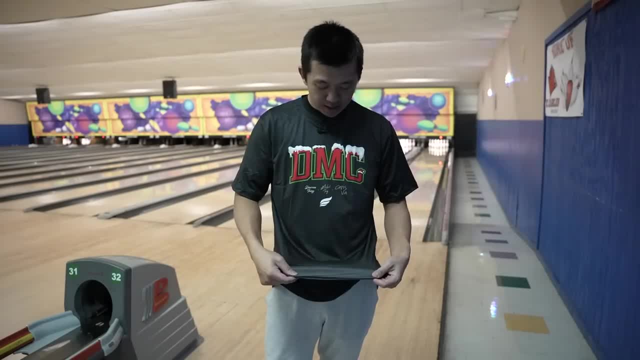 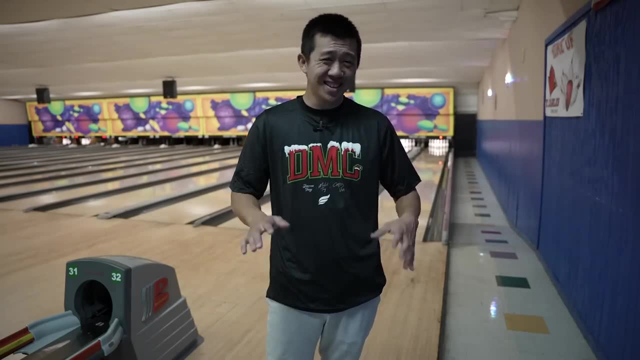 of our previous drop, our late summer drop, And let me tell you this new clothes. we've got a different material, a lot stretchier. I know the first drop of hoodies a little stiff. These ones super stretchy, super comfortable.